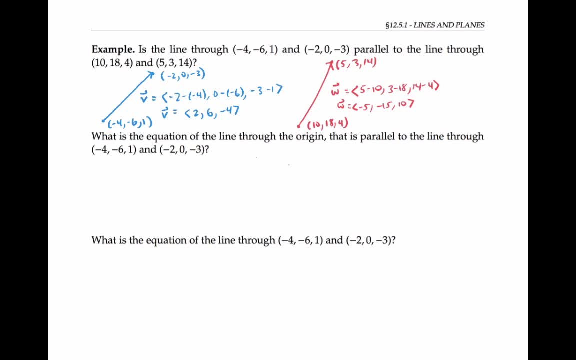 multiple of w. In fact it's easy to check that v is negative two fifths times w, And so the two lines are indeed parallel. Now suppose I want the equation of a line through the origin That's parallel to the line through these two points, So that's a line in space that 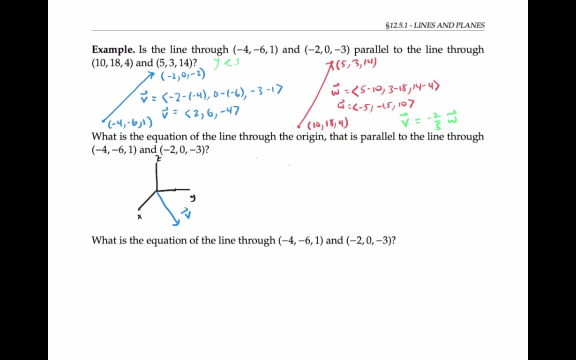 heads off in the direction of v. So if I place v, like I have done with its tail end, at the origin, then the point at the tip of v, so that's the point to six, negative four, will be on my line, So will the point halfway along v, that would be the point one. three negative: 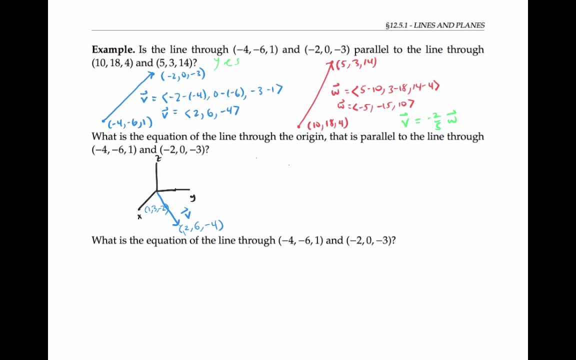 two And the point at the tip of two v, that would be the point 412 negative eight, will also be on my line. In fact, any point with coordinates two t 60 negative 40 will be on my line. that would be the point at the tip of the vector t times v, In other words the 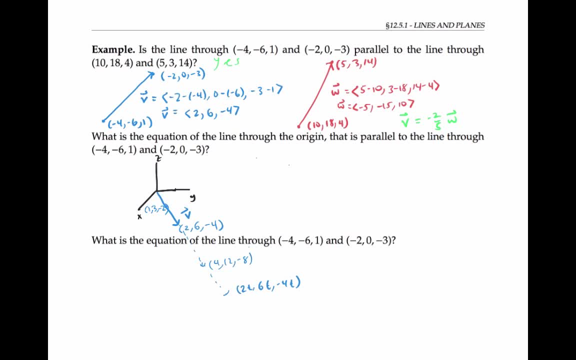 line through the origin that is parallel to v will consist of all points of the vector form: x equals two, t, y equals 60. And z equals negative 40, where t is a real number. Notice that negative values of t correspond to points on this end of the line. Now, that was the 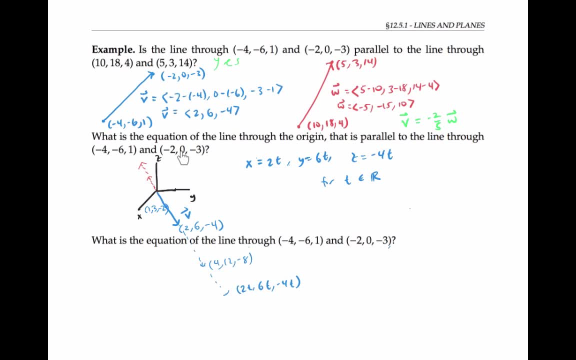 line through the origin that was parallel to the line through these two points. Next, let's find the equation of the actual line through these two points. This line will also be parallel to v, But I'll have to be shifted off the origin to go through these two points. For example, 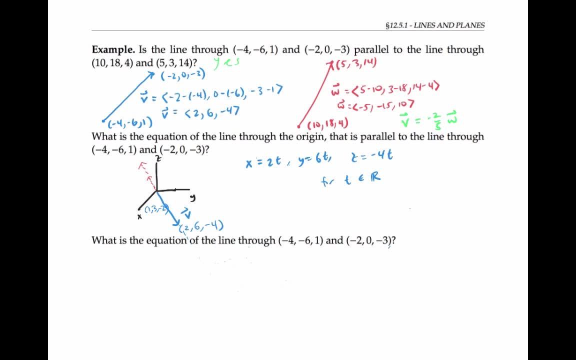 if I focus on this point, then I see that the line will have to be shifted to go over in the x direction by negative four, down in the y direction by negative six and up in the z direction by one. So it'll look something maybe like like this: Algebraically we can: 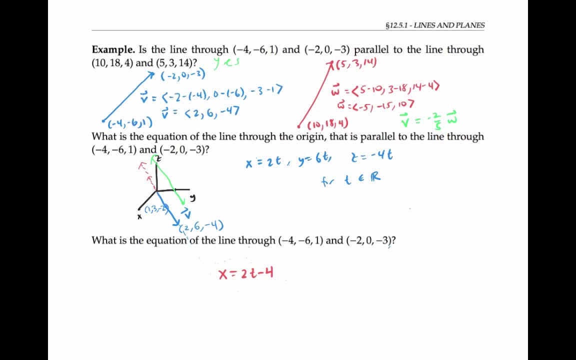 do that shifting by just subtracting four from the x values, subtracting four from the y values, subtracting six from the y values and adding one to the z values. To summarize, if I want a line through the origin that goes parallel to a vector v, I just multiply my. 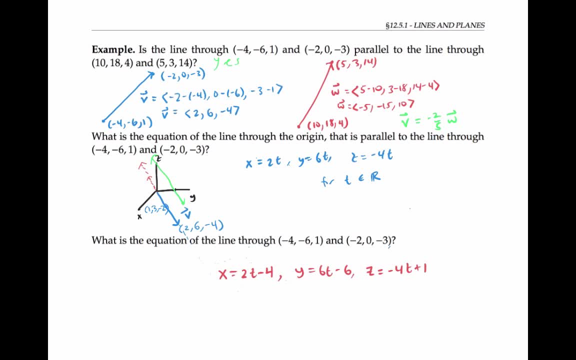 components of v by the variable t, And if I want a line parallel to v that goes through a particular point, I do the same thing and then add the coordinates of that point. Of course I could have used the other point And I would have gotten another set of equations that's in fact equivalent to the first set. 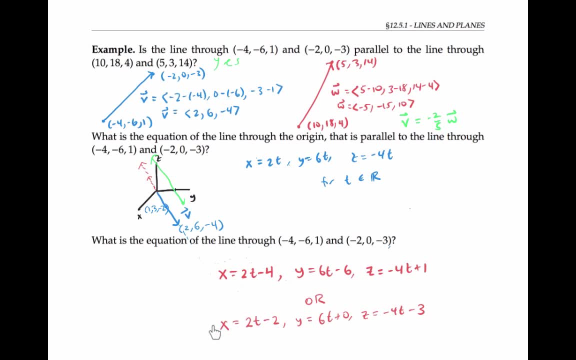 of equations To see that these two systems of equations define the same line. we can just call the second variable s instead of t and then make the substitution s equals t minus one. In other words, plugging in t minus one for s here gives us the following: 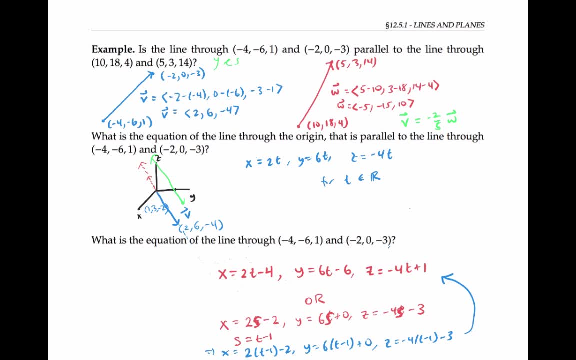 which, after a little bit of algebra, reduces to t minus one, The first system of equations. These systems of equations are called parametric equations. for the line, The parameter is t And physically we can think of this as a particle moving along a line: t describing the time, and x, y and z describing the position of that particle. 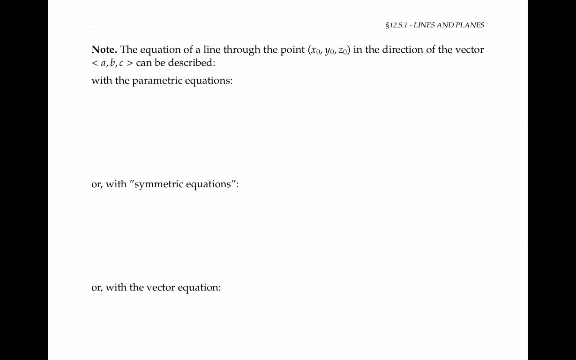 at time t. More generally, if we want to describe a line through a point- x naught, y naught, z naught- in the direction of the vector ABC, we could describe it with the parametric equations: x equals at plus x naught, y equals. 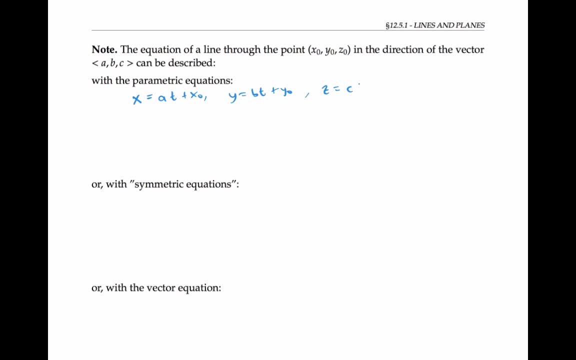 b t plus y naught and z equals c t plus z naught. Remember, if x naught, y naught, z naught weren't there, then our equations would just describe a point at the tip of a vector. t times our original vector, But by adding x naught, y naught and z naught, we've shown. 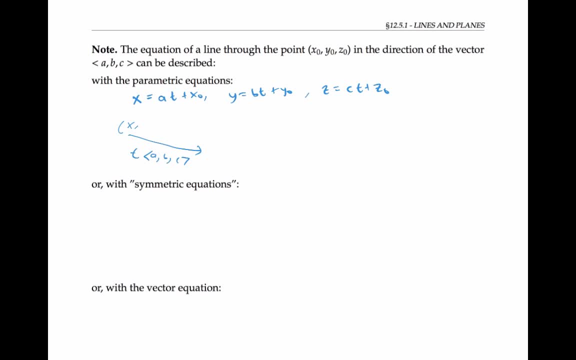 that we've shifted that line over. So there's all. go through the point: x naught y naught z naught. Now if we take our parametric equations and solve for t, we get: t equals x minus x naught over a. T equals Y minus Y naught over B, and T equals z minus z naught over C. And 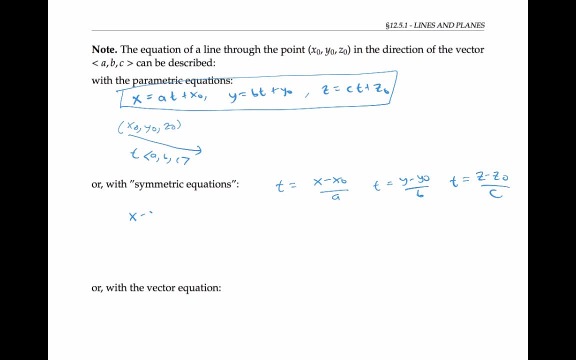 now, if we set these expressions for T equal to each other, we get: X minus X. naught over a equals y minus y. naught over C over B equals z minus z naught over C. The equations in this format are called the symmetric. 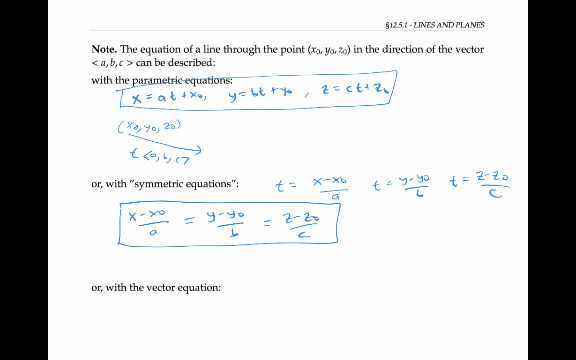 equations for the line. Finally, we can describe the line with a vector equation. R is a vector that's a function of T, whose components are given by: at plus x naught, b, t plus y naught, CT plus z naught. The vector equation is very similar to the parametric equations Geometrically. 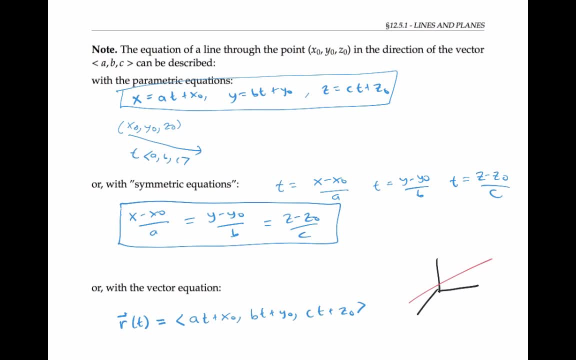 we think of our line going through space, and a point on the line whose coordinates are given by the parametric equations can also be thought as the tip of a vector starting at the origin. So this we can think of as the vector r of t, Physically, as we think. 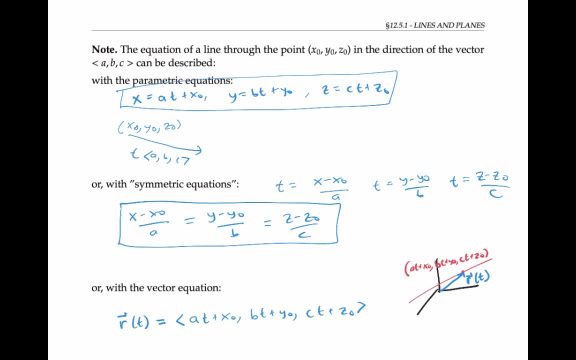 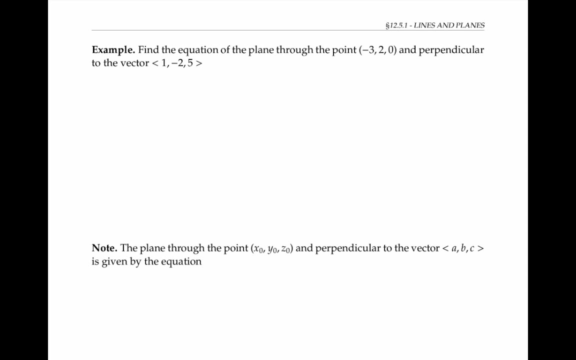 of a particle moving along the line over time. we can think of a vector with its or its tail at the origin, sweeping along that line, with its tip always on the line. We've looked at equations for lines. Now let's take a look at equations for planes. Suppose we want to find the equation of a plane through. 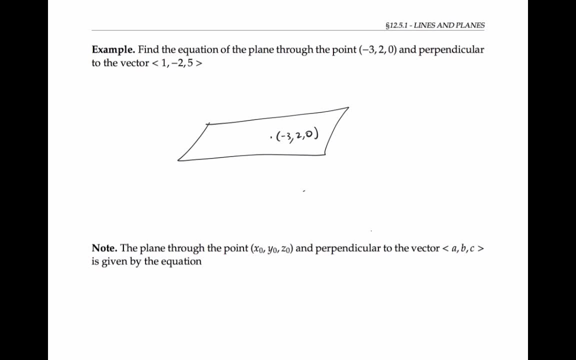 the point negative 320 and perpendicular to the vector with components one negative 25.. I'll call that perpendicular vector v. Now if I take any point x, y, z on my plane, then the vector from the given point to the point x y z has to be perpendicular to my vector. 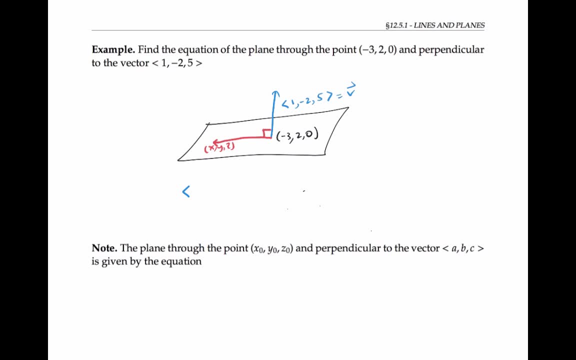 v In terms of dot product. that means the vector x minus negative three, y minus two, z minus zero dotted with the vector v is going to have to be zero. Rewriting: I get the equation one times x plus three minus.